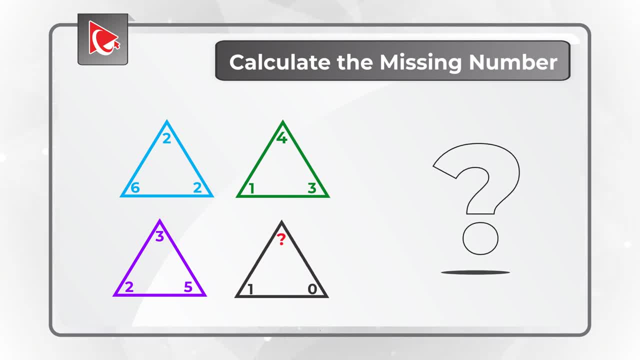 there is a missing number which you need to calculate based on the four different choices: Choice A: 0.. Choice B: 1.. Choice C: 2. And Choice D: 3.. Do you see the answer? Let me give you a hint. 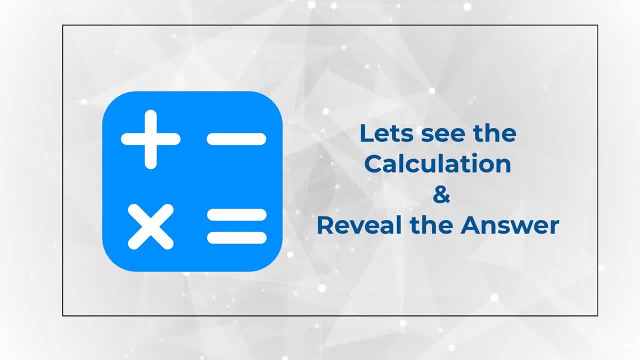 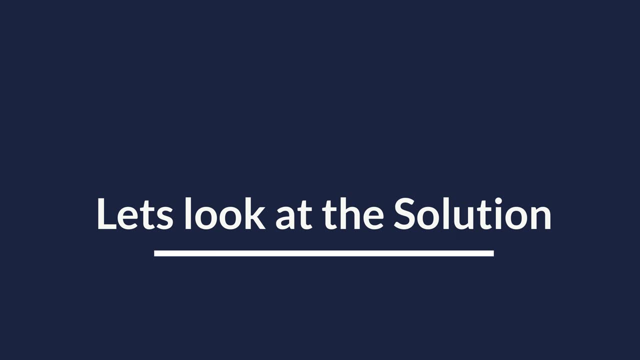 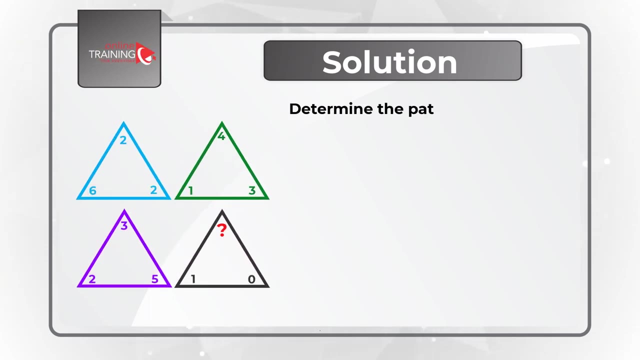 There is a true calculation and not guessing behind determining what the number is Ready or not. I am going to move forward and reveal the solution to you. As I mentioned, the trick about this problem is that the number can be calculated, And the key to calculate it is to determine the pattern. 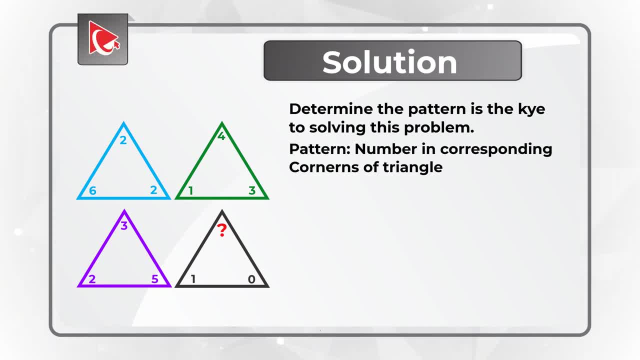 And then the pattern here is that the numbers in the corresponding corners of the triangles all add up to 10.. Let's do the math and start with the black triangle, The bottom-left corner. 6 plus 1 plus 2 plus 1 equals 10.. 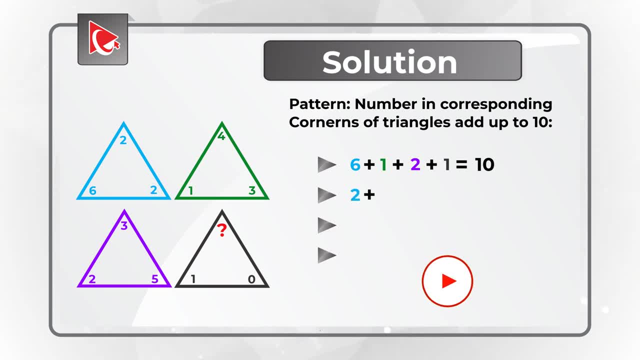 Let's go to the bottom-right corner of the triangle: 2 plus 3 plus 5 plus 0 is also 10.. And now, in the same way, let's do the math and calculate the missing number: 2 plus 4 plus 3 plus equals 10.. 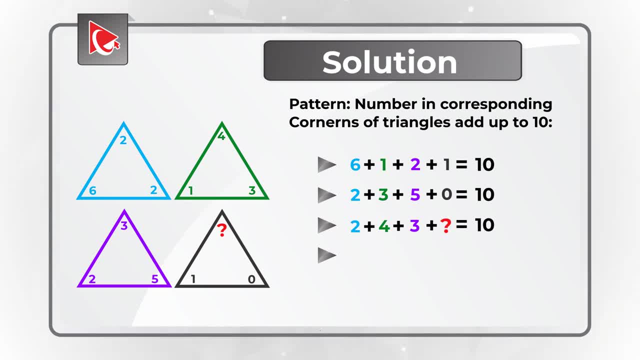 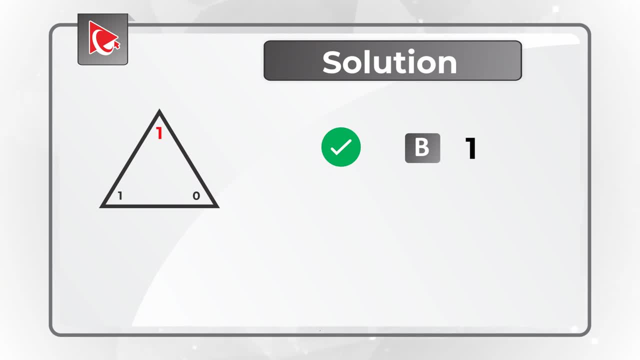 Based on these calculations equals 1.. So the correct choice here is choice B 1.. Keep in mind that sometimes, in these types of problems, triangles are colored And the only reason this is done is to confuse you. to look for the patterns inside the triangles itself. 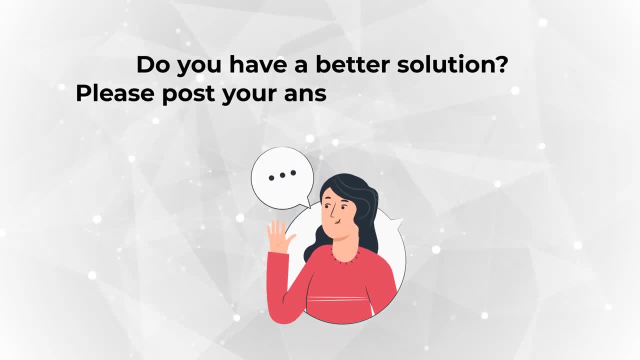 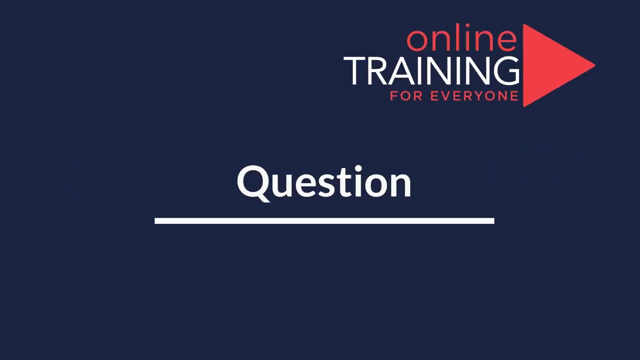 I truly hope that you've nailed this question on your own or learned how to answer similar problems on the test Very frequently on the test. you need to identify the problem. You need to identify words with the similar meaning. In this case, you're presented with 5 words. 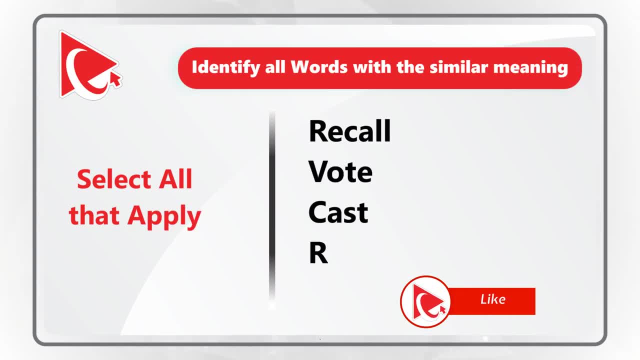 Recall, Vote Cast, Remember and Remind Which words on the list have a similar meaning. Very interesting question, because the number could be between 2 and 5.. Did you get to the answer? Let's move forward and I'll share with you the correct solution. 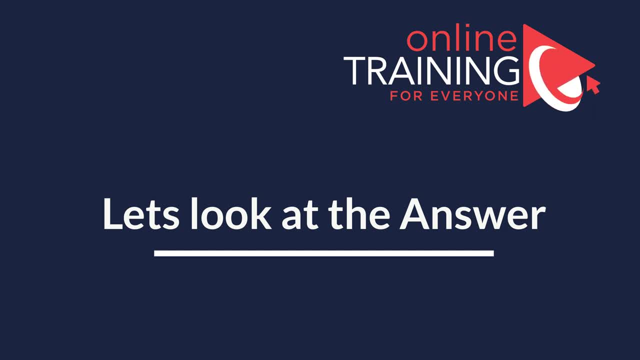 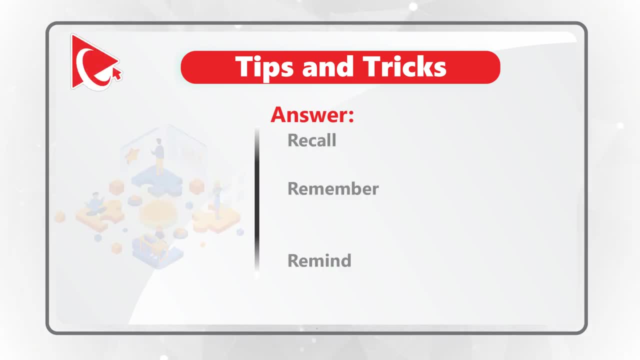 From my standpoint, there are 3 words here with the similar meaning And obviously, if you disagree, feel free to share your feedback in comments. But I see words Recall, Remember and Remind having similar meaning in this particular question To understand why we need to look at the definition. 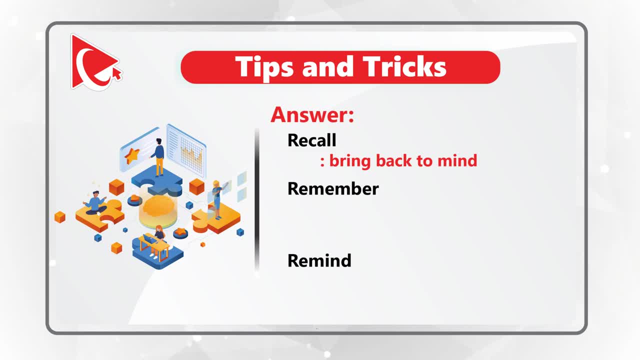 For example, word Recall means bring something back to your mind, Word Remember means bring forward past memory into the present And word Remind means cause someone to remember someone or something. Not the easiest question, because each word can have multiple definitions and multiple meanings. 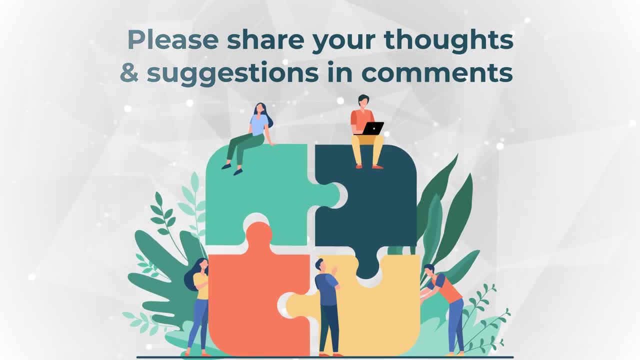 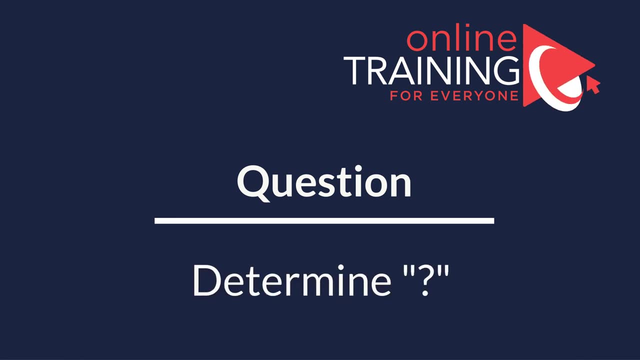 And to solve it you need to know all of them and connect them to get to the final answer. I love this question because you need to determine relationship between the shapes And you need to determine which shape has similar relationship to rectangle If you take a close look. 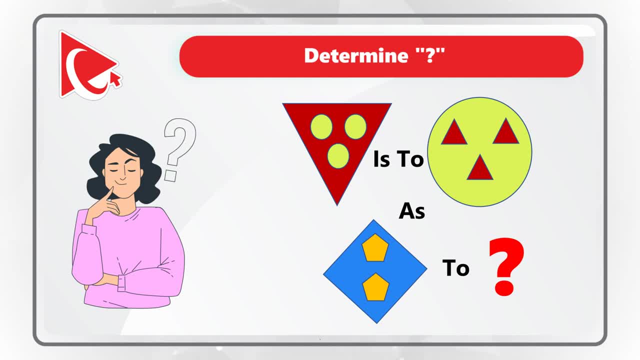 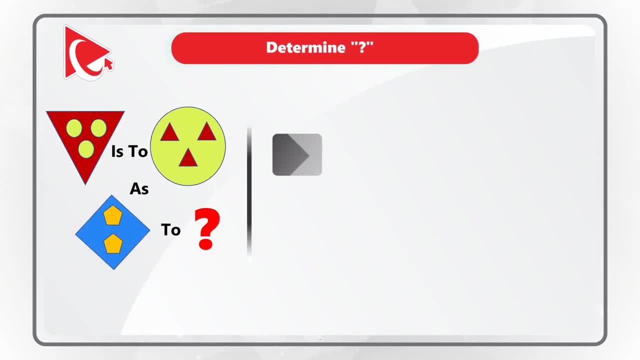 you will see that there are other smaller shapes inside the larger shapes And you have 4 different choices to choose from the final answer: Choices A, B, C and D. Take a close look to see if you can come up with the answer. 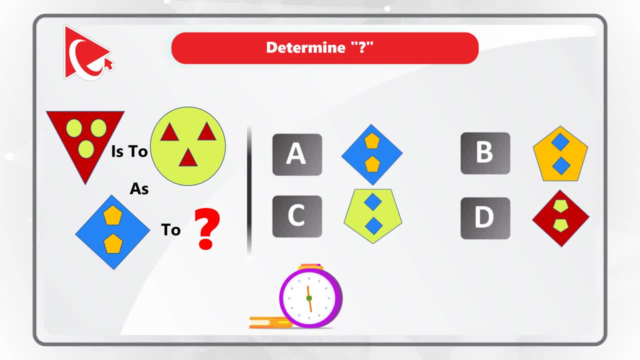 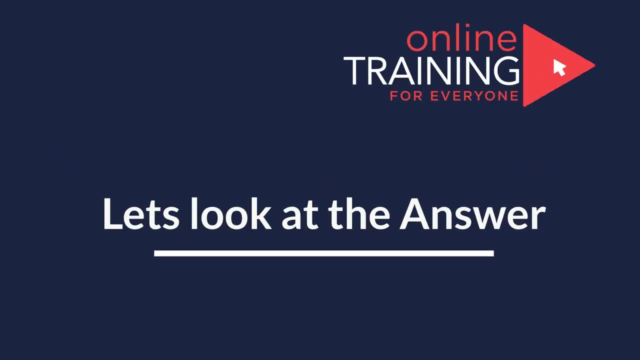 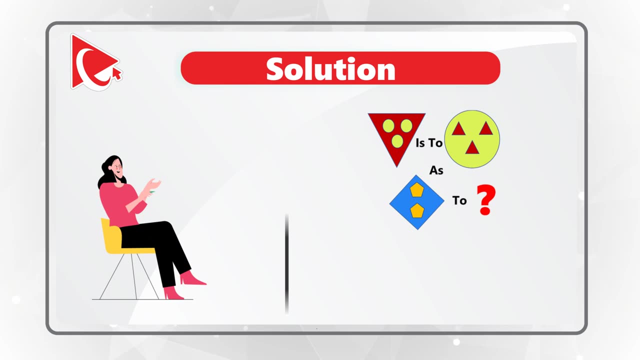 Have you tried solving it? Were you successful? Let's move forward so we can get to the correct solution together. To determine the correct answer in this case and in a lot of other cases, you need to look for patterns, And the pattern in this particular case is that, to build the relationship, inside shape becomes outside shapes. 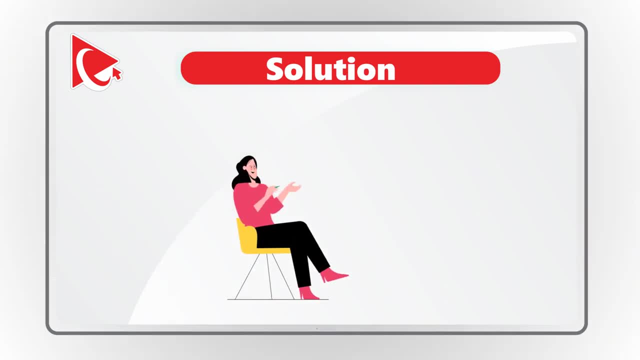 preserving the number of the inside to outside shapes ratio. If you look closely at the relationship presented in this question, you see that the red triangle has green ovals inside And it has a relationship to green oval that has red triangles inside. Knowing this, 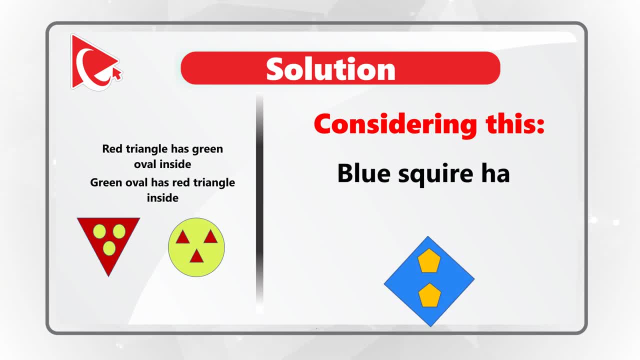 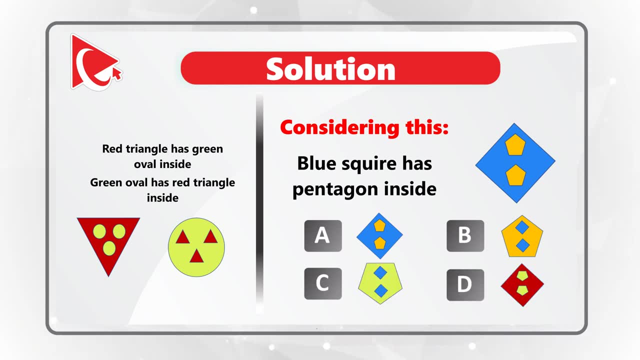 we need to determine relationship of the blue square that has pentagons inside to one of 4 shapes presented in possible answers. Do you see it now? All you need to do in this particular answer is to take the pentagon which is inside the square. 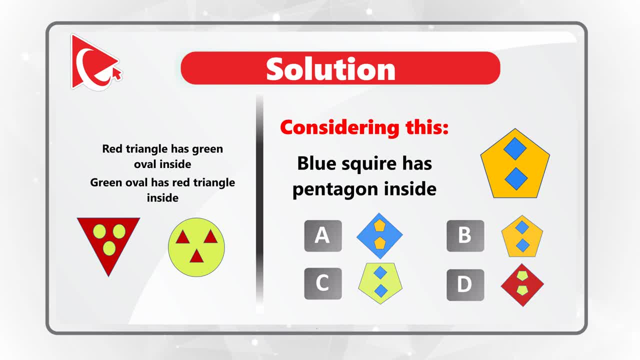 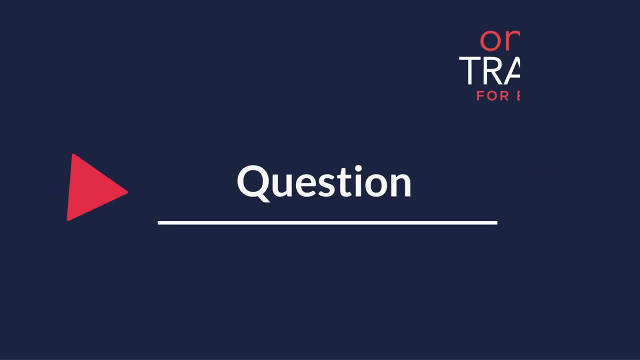 enlarge it and put blue squares inside. So, as you might have guessed, the correct answer here is choice B. Hopefully you've nailed this question on your own and now know how to answer similar problems on the test. Here's the practice problem for you. 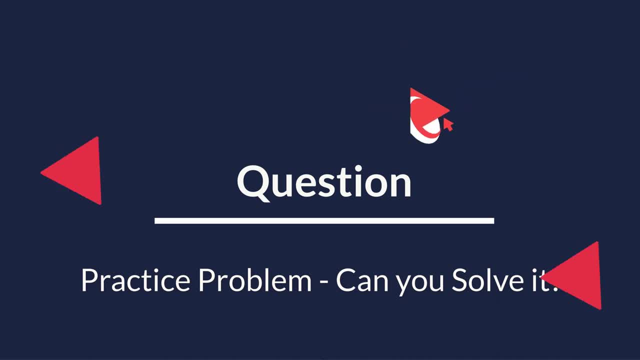 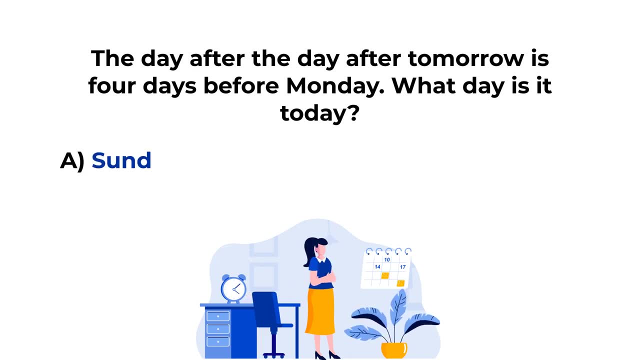 The day after the day after tomorrow is 4 days before Monday. What day is it today? You have 4 different choices: Choice A – Sunday. Choice B – Monday. Choice C – Friday. Choice D – Saturday. Feel free to pause this video to see if you can come up with the solution. 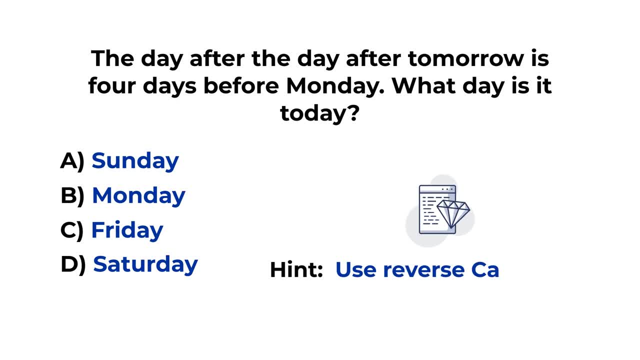 I would like to give you a hint. The best way to solve these types of problems is using reverse calculations. So do you see the answer? Give yourself 10 to 15 seconds to see if you can come up with the solution. Did you figure out the answer? 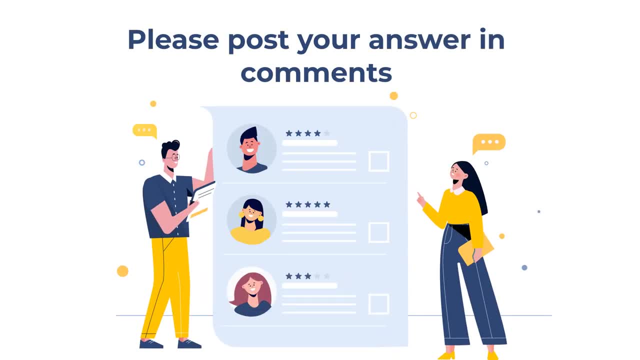 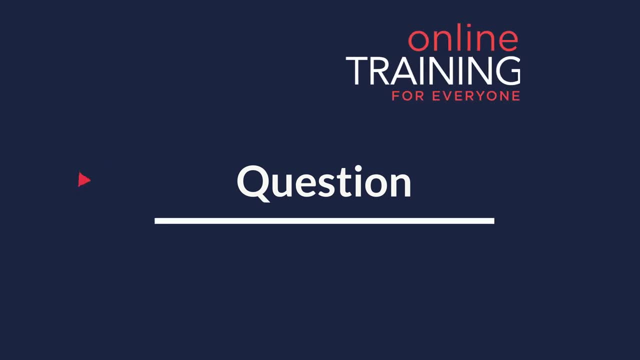 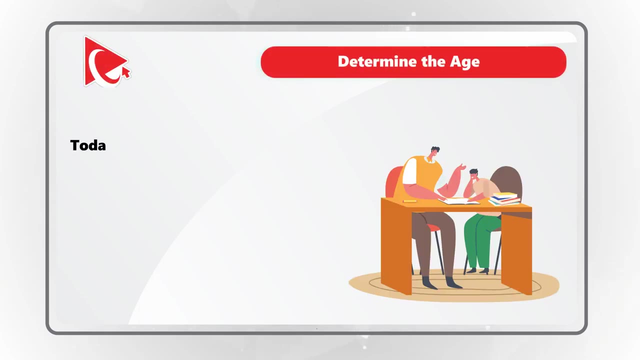 Make sure to post your answer, as well as your rationale for solving this problem, in the comment section of this video. Thanks for participating and good luck. Here is the frequent test problem where you need to determine the age of the family members. Today, a father is 3 times as old as his son. 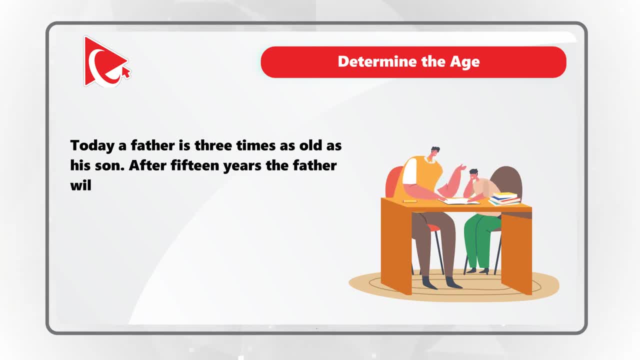 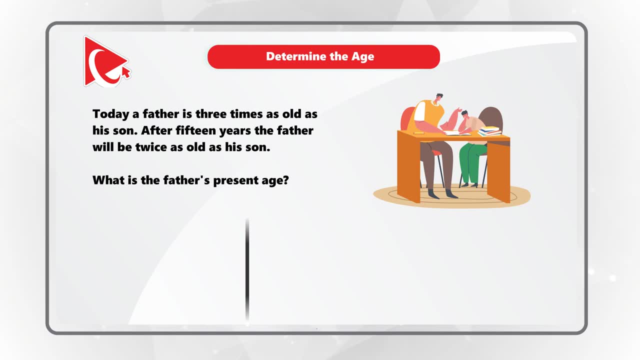 After 15 years, the father will be twice as old as his son. What is the father's present age? And you have 4 different choices: Choice A – 40 years. Choice B – 45 years. Choice C – 50 years. 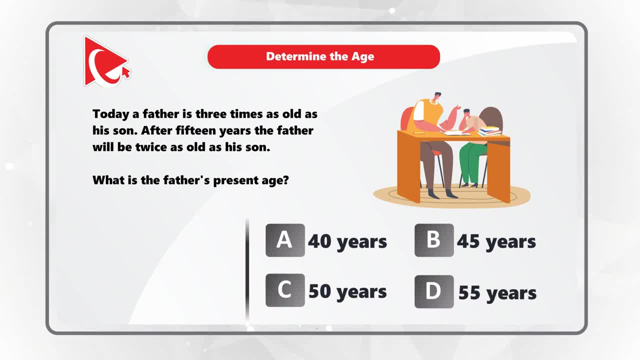 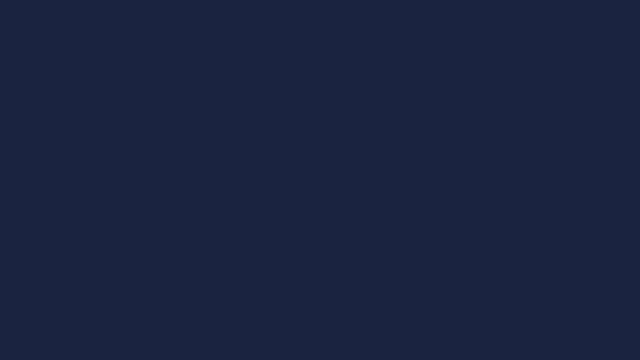 And Choice D – 55 years. Do you see the answer? Give yourself a little bit of time to see if you can come up with the solution. One of the ways to solve this problem is to take the number from the solution and see if it will work. the math: 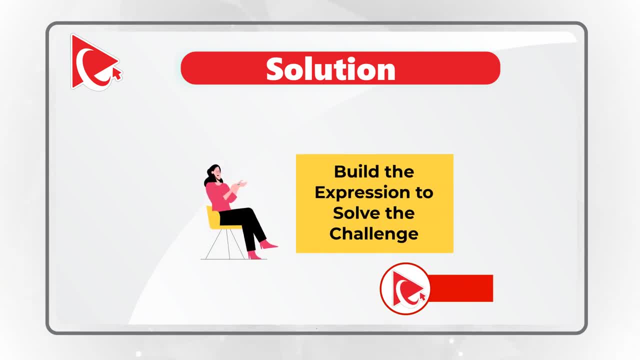 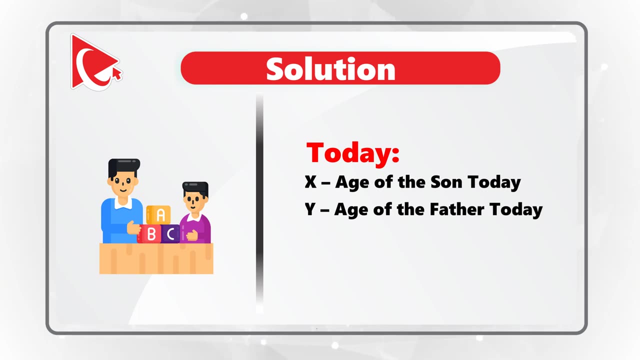 But instead of doing that, we are going to build the expression and calculate the father's present age. In the first step, we are going to introduce two variables: Variable X will represent age of the son today, and variable Y will represent father's age today. 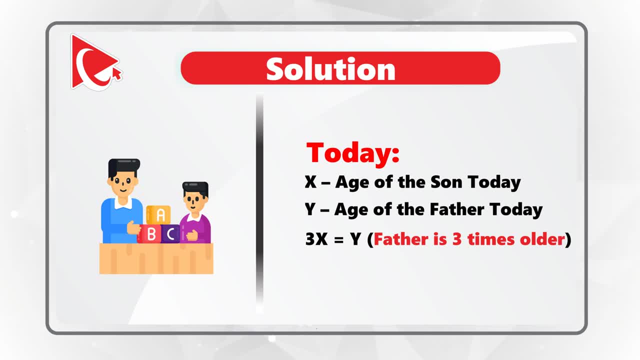 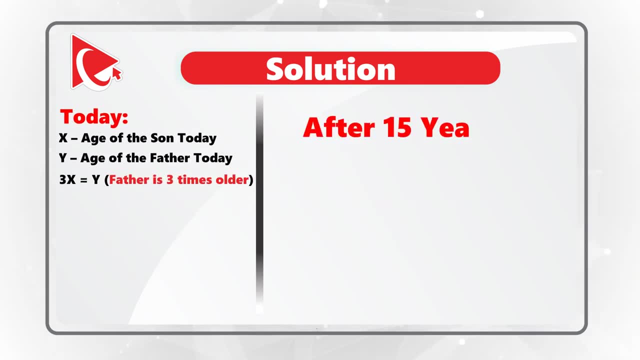 So our first formula is 3X equals Y, which indicates that today, father is 3 times older than his son. After 15 years, our expression will be different. The new expression will be Y equals 2X plus 15.. Because in both cases Y is the same. 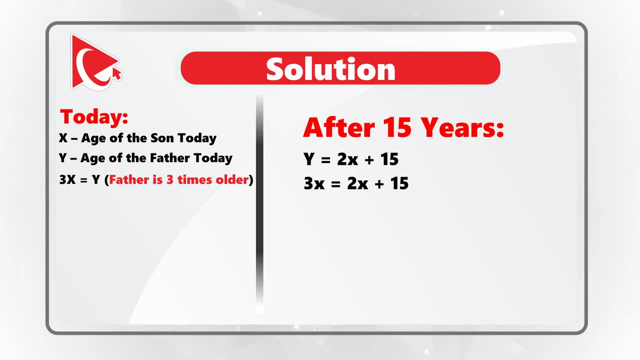 we can build a new expression: 3X equals 2X plus 15.. Once we simplify, 3X minus 2X will equal 15.. And, after completing the calculations, X will be 15.. Y will be equal 15.. 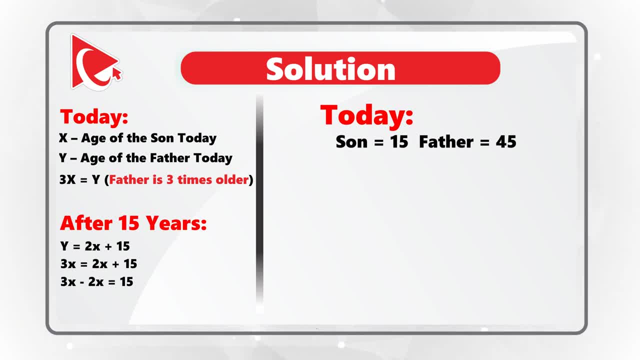 And Y will be equal 45.. Based on this, today's age of the son is 15 years old, Which means that after 15 years, son will be 30 years old and father will be 60 years old. Hopefully you've nailed this question. 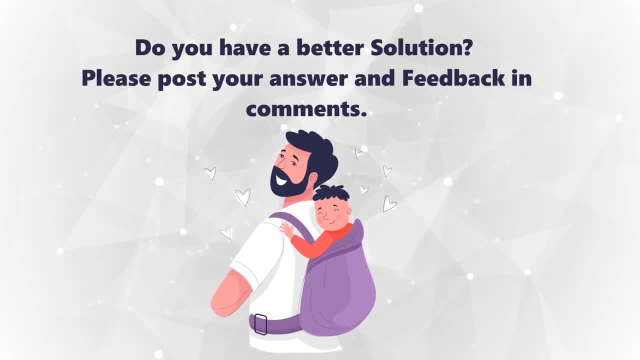 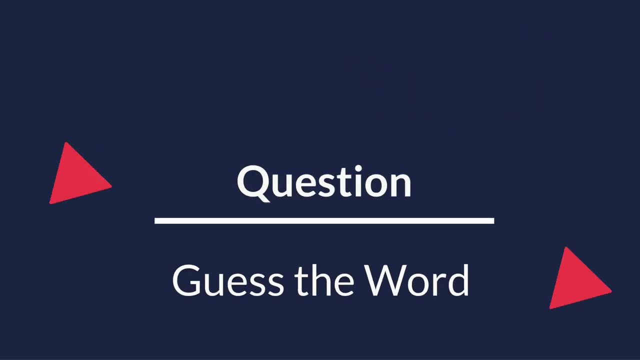 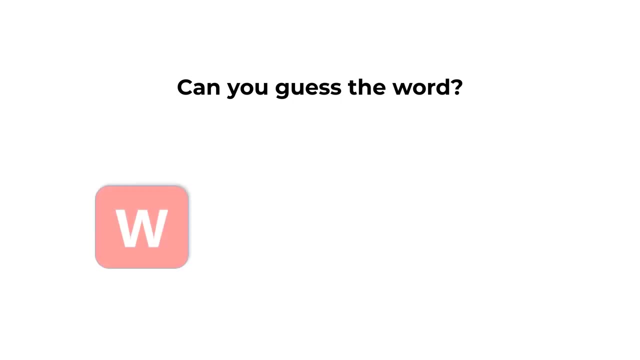 and now know how to answer similar age problems on the test. Here's the cool question that you frequently get on the test. You are presented with four different letters and you need to guess the word using all letters presented. The letters we have are W, O, B and L. 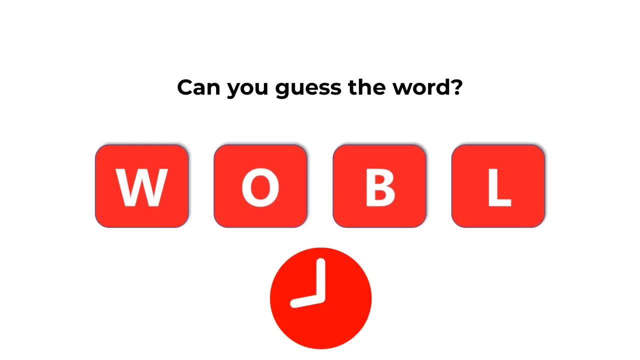 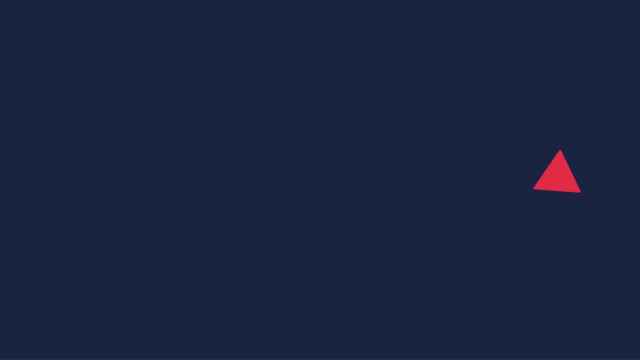 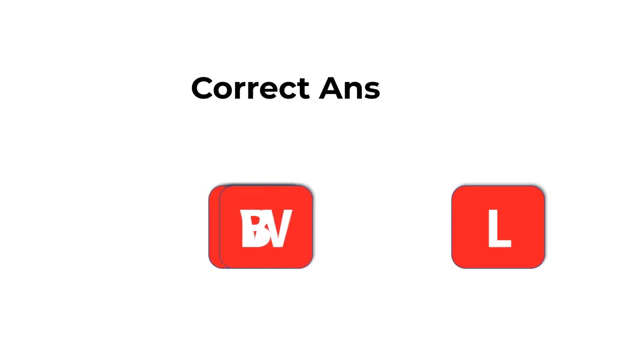 Can you guess the word? Give yourself 10 to 15 seconds to see if you can come up with the answer. Ready or not, let's go ahead and reveal the solution. The correct answer here is BALL, which is spelled as B, O, W and L. 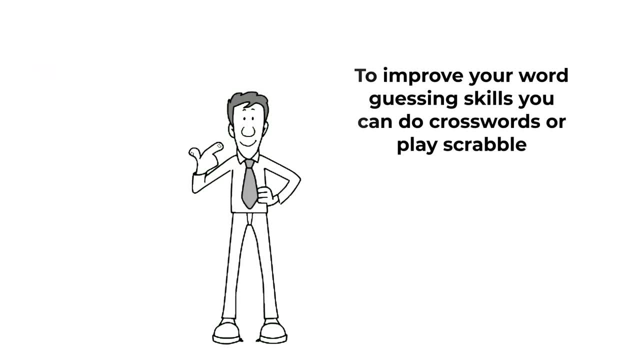 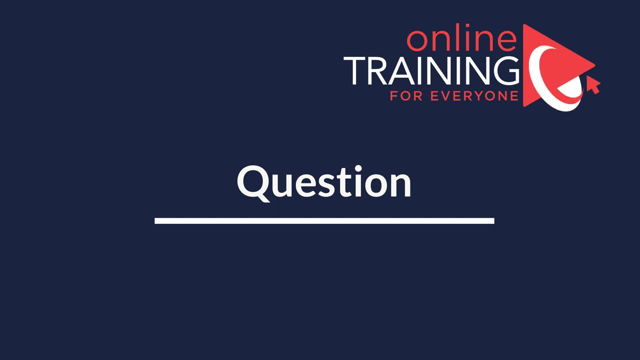 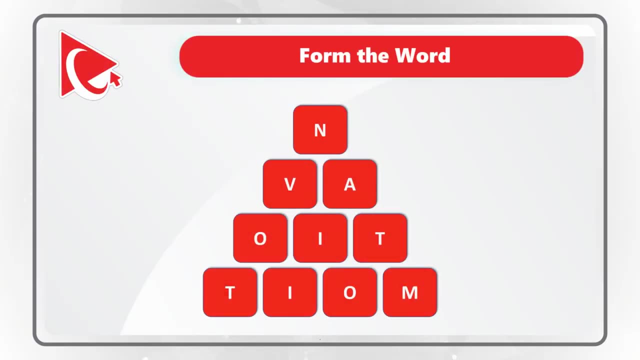 Hopefully you've nailed this question and now know how to answer similar problems on the test. One of the very hard challenges is forming the words using certain number of letters of the English alphabet. In this question, you are presented with 10 letters and you need to form the word using all the letters only once. 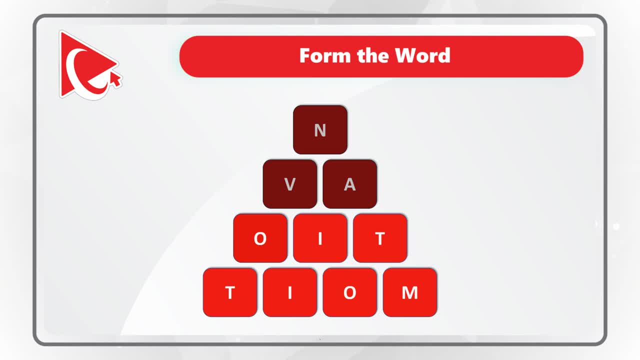 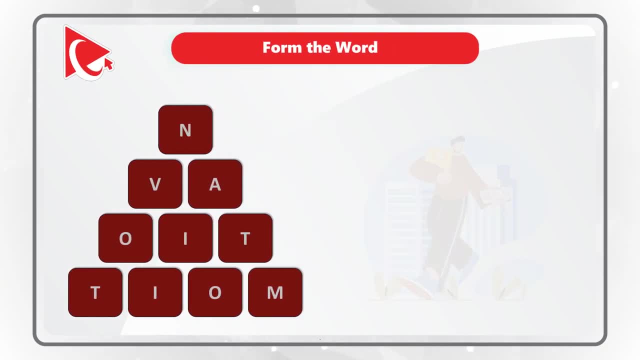 The letters are N V A O I T and T I O M. Do you see the word here? Give yourself a little bit of time, maybe 20 to 30 seconds. Hopefully you solved it because I am moving forward. 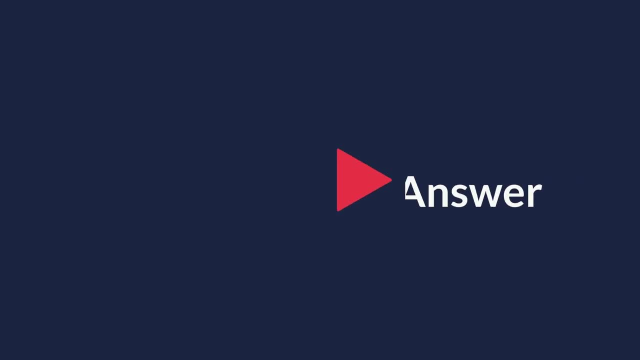 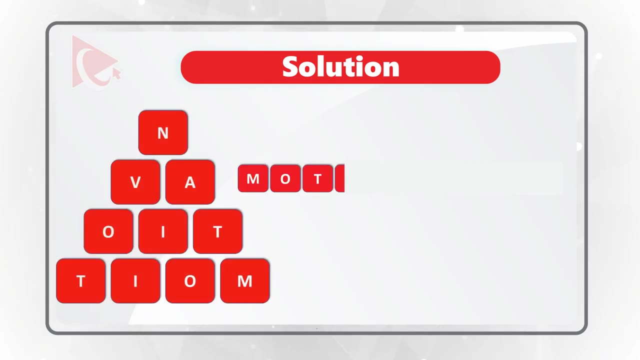 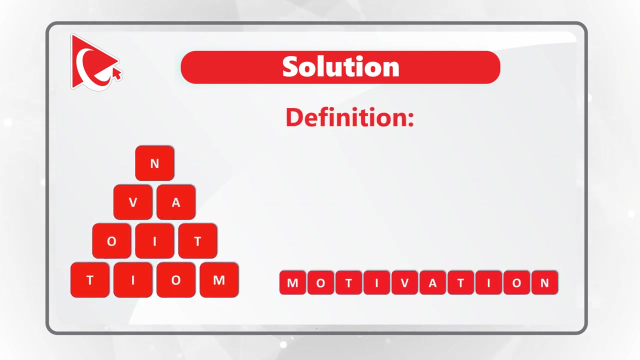 and revealing the solution. As you might have guessed, the word is MOTIVATION. Let me spell it for you: M O T I V A T I O N, And the definition of the motivation is that. 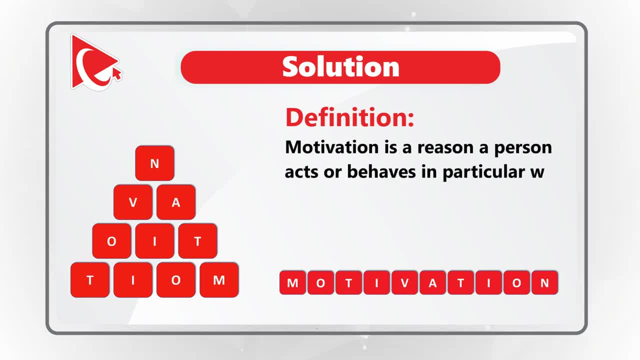 motivation is a reason a person acts or behaves in a particular way. It is also a process that initiates, guides and maintains goal-oriented behaviors. Believe it or not, but doing more practice exercises helps you get better with the skill of forming the word. 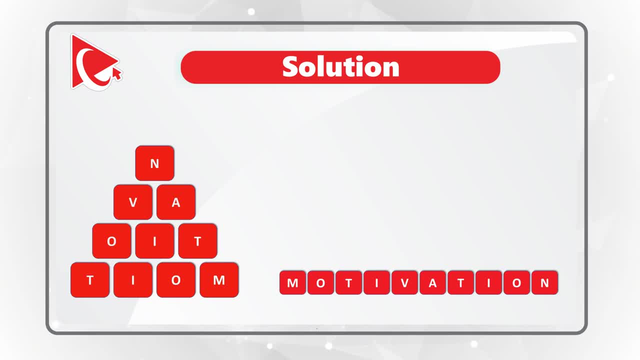 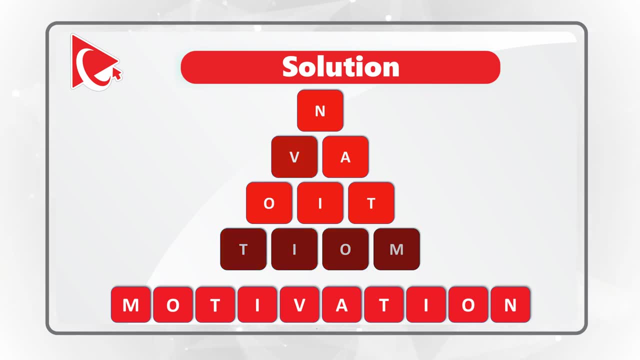 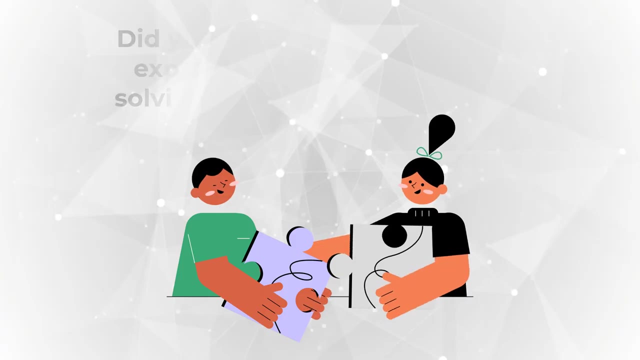 For example, if you start with the bottom right corner, you can form the word MOTIVATION. You see M-O, and then you swap T-I and then, if you continue, you go V-A, T-I-O-N. You can solve these types of challenges better. 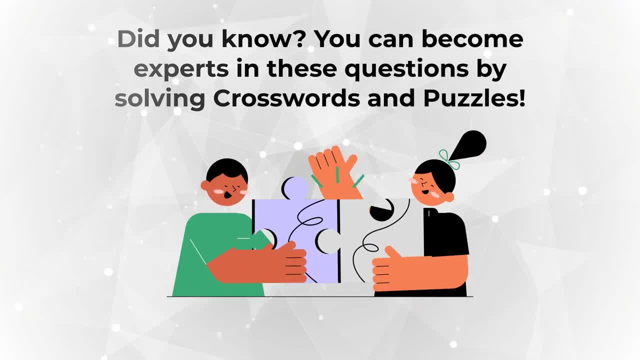 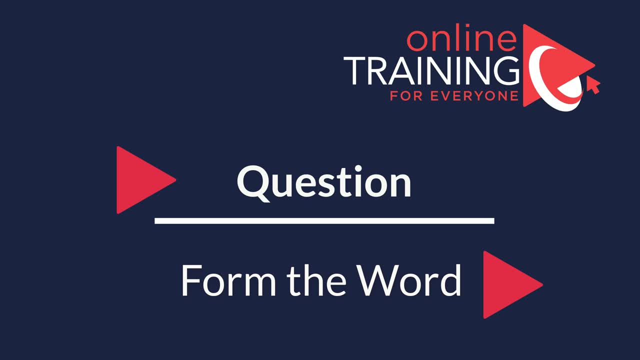 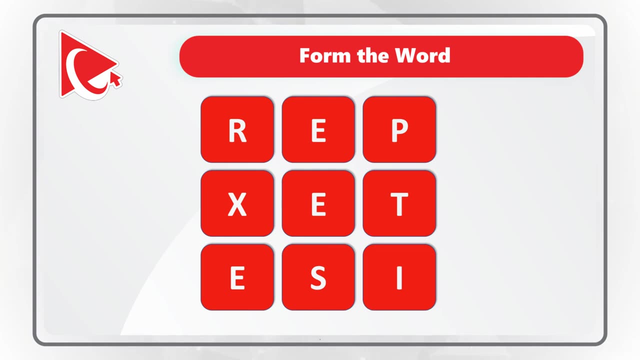 if you do more crosswords and puzzles Very frequently, you might get tested on how quickly you can form the words using letters of the English alphabet. In our case, you are presented with 9 letters and you need to form the words using all the letters only once. 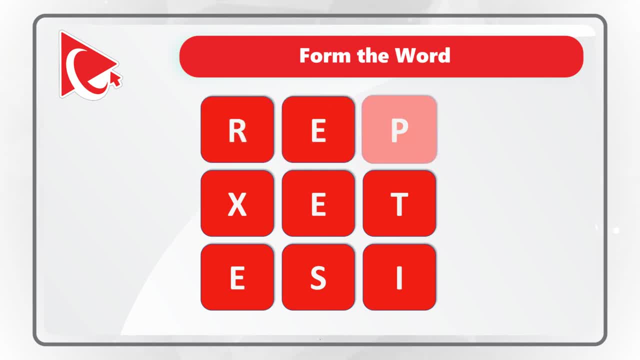 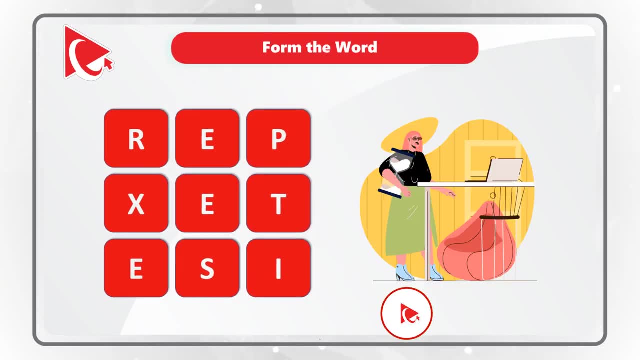 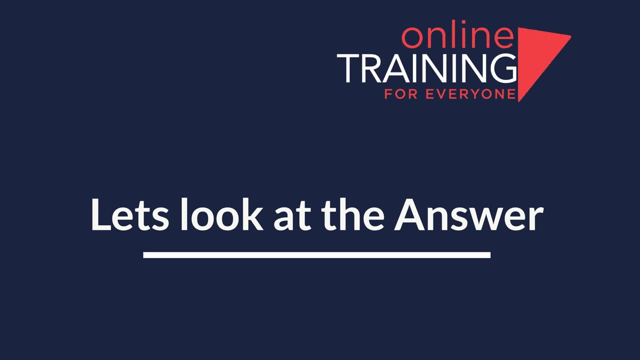 The letters are R-E-P-X-E-T-E-S-I. Do you see the word? Give yourself a little bit of time, maybe 10 to 15 seconds, to see if you can answer the question Ready or not. I am going to reveal the answer. 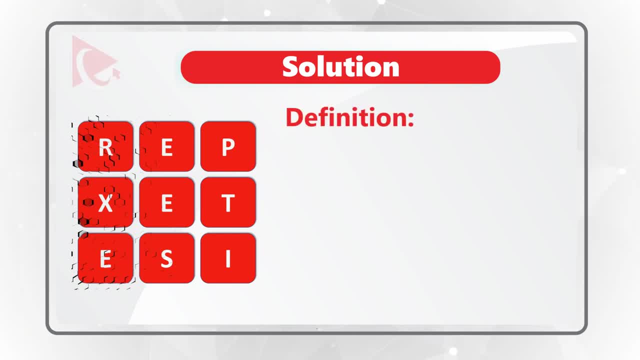 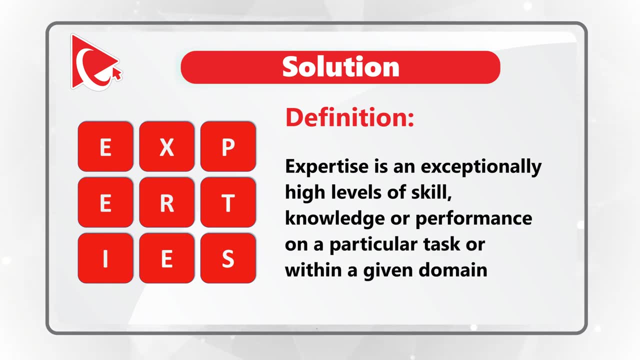 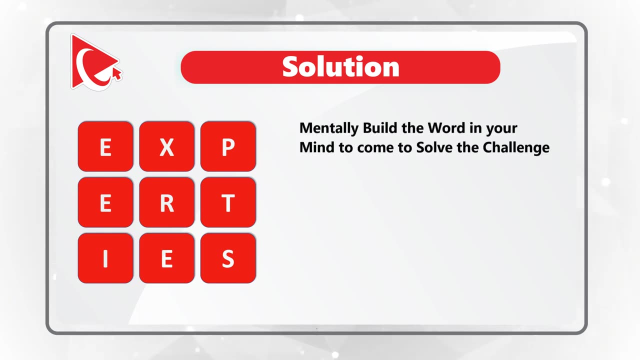 which is the word EXPERTISE, And the definition of expertise is an exceptionally high level of skills, knowledge or performance in a particular task or within a given domain. To better solve these types of challenges, try to look at the presented letters and try to form the word. 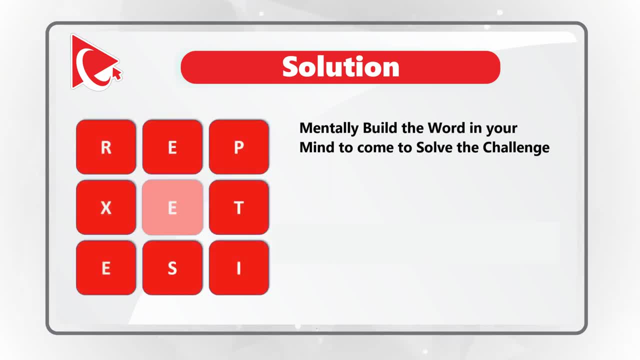 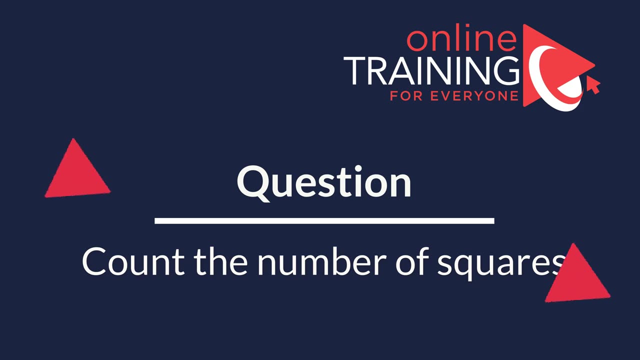 For example, if you start in the middle and go E-X-P-E-R-T-I-S-E, you can definitely form the word EXPERTISE. Here is an interesting problem where you need to count the number of squares in the presented shape. The correct number is one of four different choices. 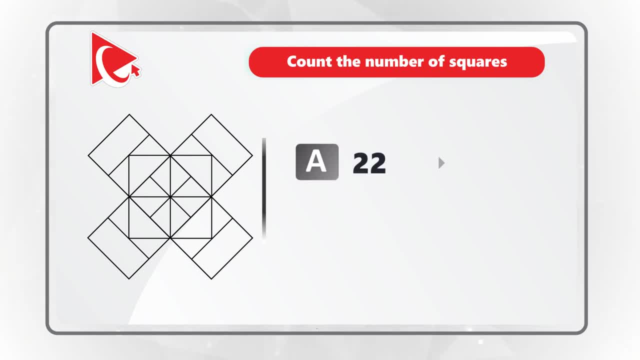 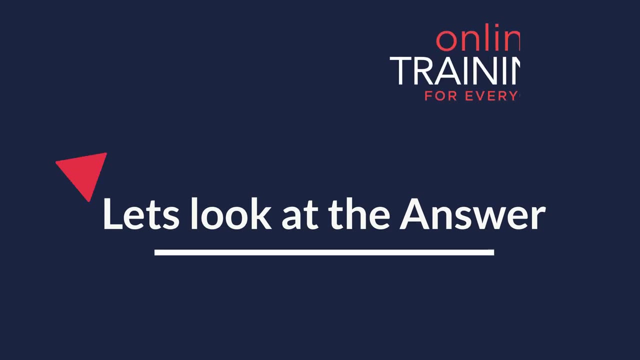 Choice A: 22., Choice B: 10., Choice C: 18. And choice D: 14.. Take a close look at the picture to see if you can come up with the right solution. I was really impressed, But there are 18 squares in this picture. 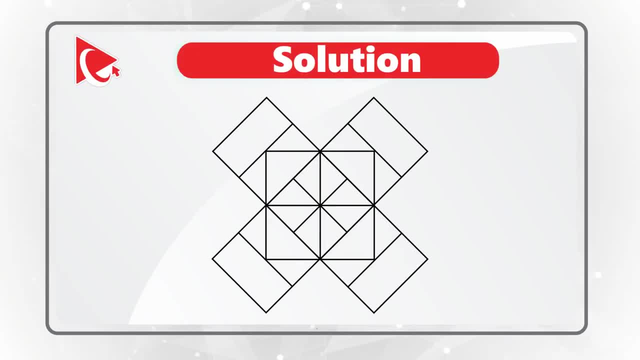 Let me show them all to you: One, Two, Three, Four, Five, Six, Seven, Eight, Nine, Ten, Eleven, Twelve, Thirteen, Fourteen, Fifteen, Sixteen, Seventeen And eighteen. Do you see any additional ones? 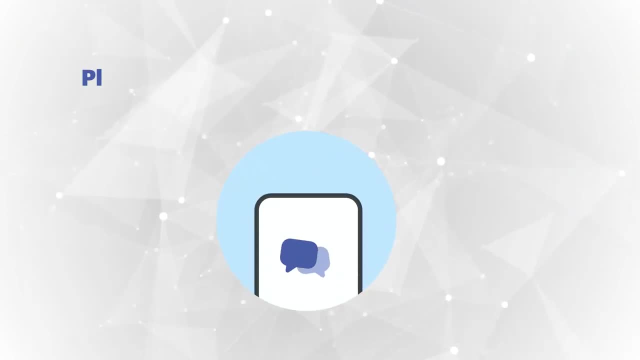 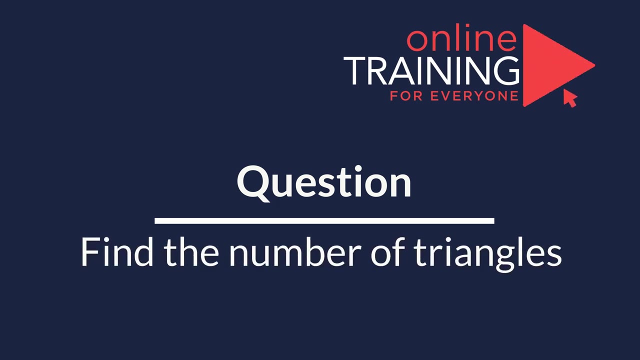 It is totally possible that I missed one of the squares, And if you do see any additional ones, please make sure to post them in comments. And now here is the question for you to try your skills. You need to determine how many triangles are shown on the screen. 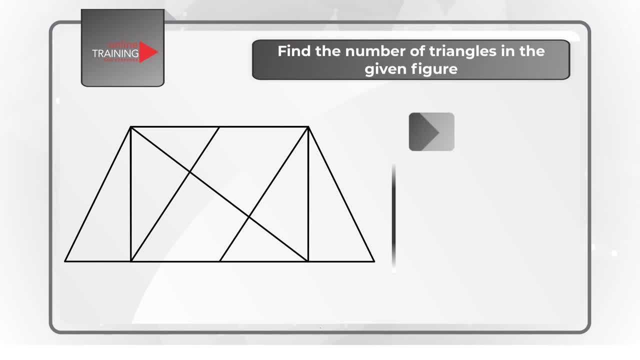 You have four different choices: Choice A: 8., Choice B: 10., Choice C: 12. And choice D: 14.. Feel free to pause this video to calculate the right answer And make sure to post your solution in comments. 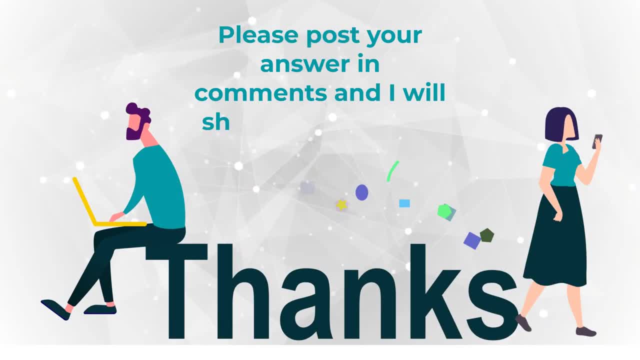 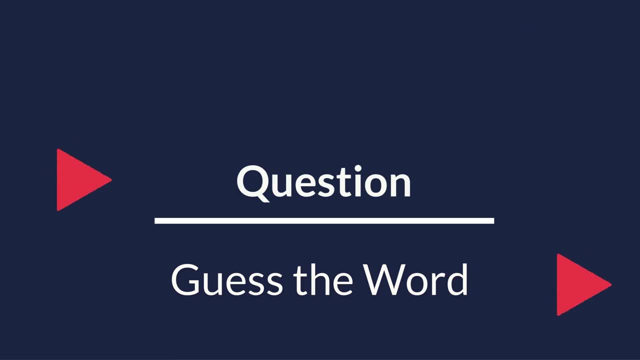 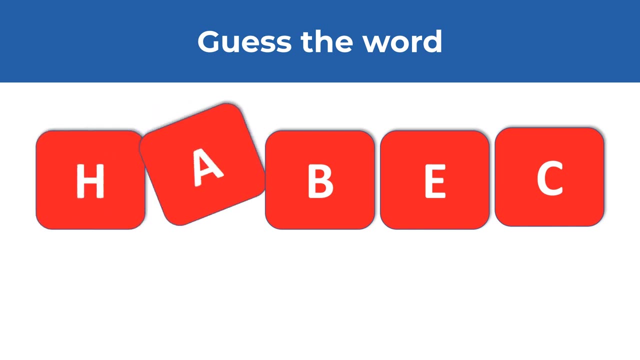 so I can give you my feedback. Thanks for participating and good luck. Here is an interesting question from the recent test. You need to figure out the word from the five letters you see on the screen. The letters are H, A, B, E and C. 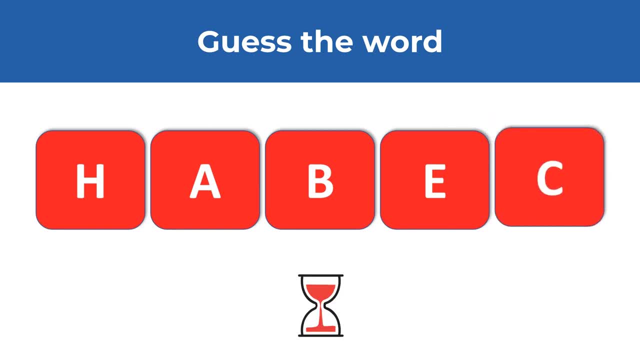 Do you see the word? Give yourself 10 to 15 seconds, maybe 20 seconds. You can pause this video to see if you can figure it out on your own. Make sure to use all the letters and make sure to use each of the letters once. 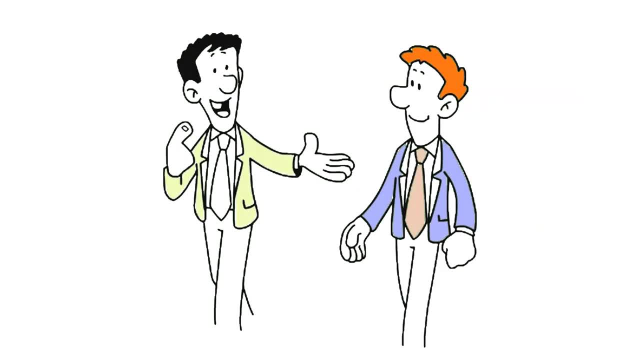 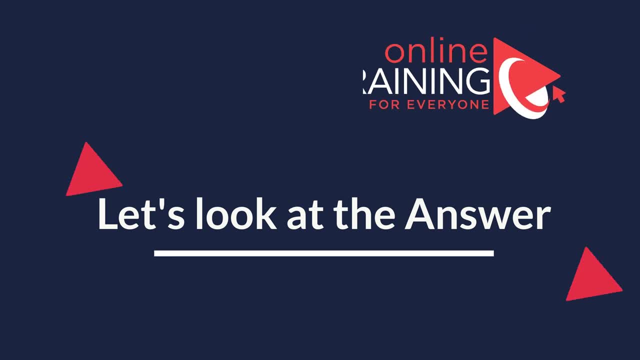 Ready or not, I am going to move forward and share with you my solution, But keep in mind that a lot of times, multiple words can be formed, So if you see another word, please make sure to share it in comments. The solution I found is the word beach. 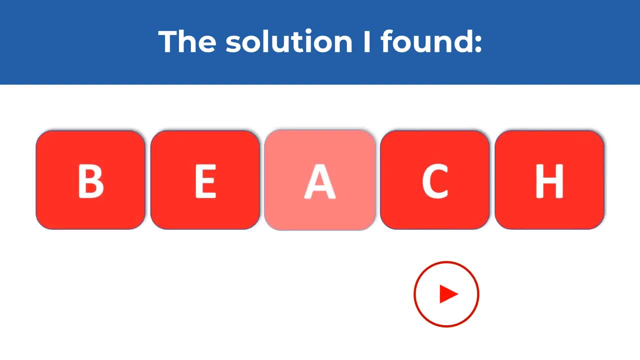 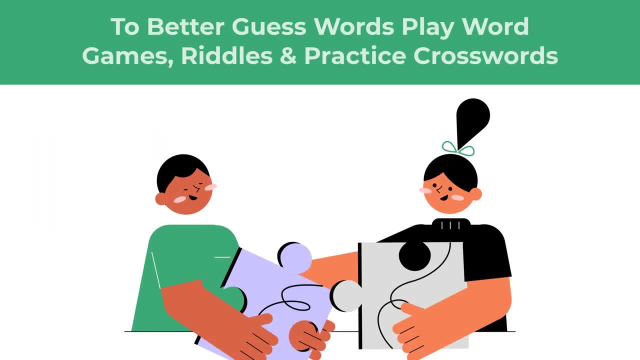 Let me spell it for you: B, E, A, C, H. Do you see any other solutions? Make sure to post them in comments, And if you'd like to improve your ability to guess the words, you can play word games. read a lot. 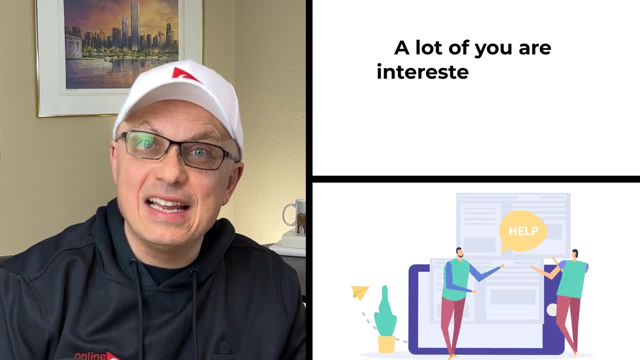 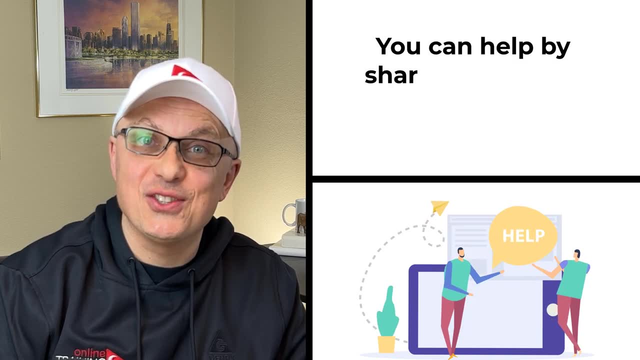 and practice crosswords and puzzles. A lot of you are interested and ask me: how can I help others? One of the ways you can help other people is by sharing the latest questions you see as part of the assessment test And when you share. 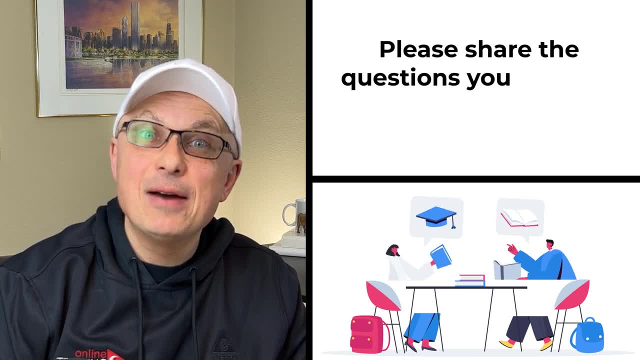 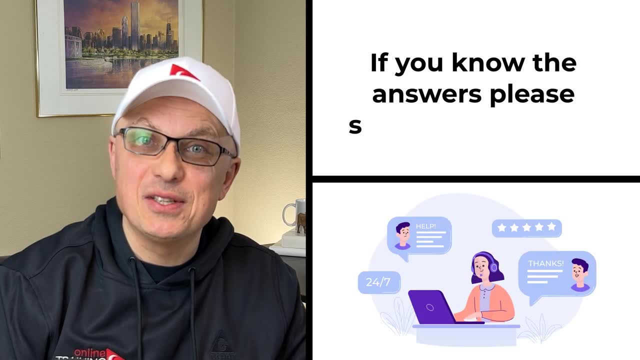 please make sure to also include how you answered them. Please share the question you recently encountered in the comments section of this video And if you know the answers, please share them as well. And now let's continue and get you ready for the test. 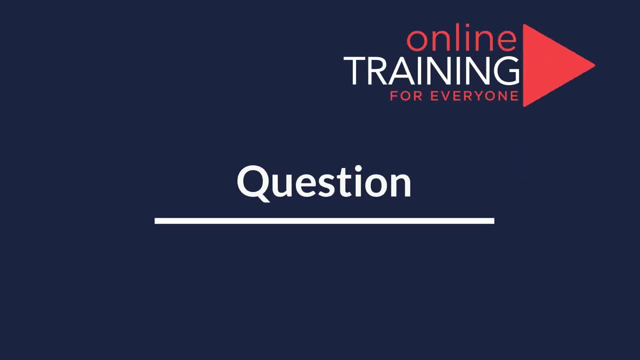 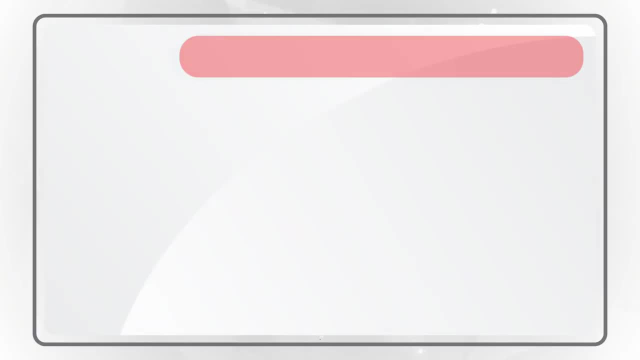 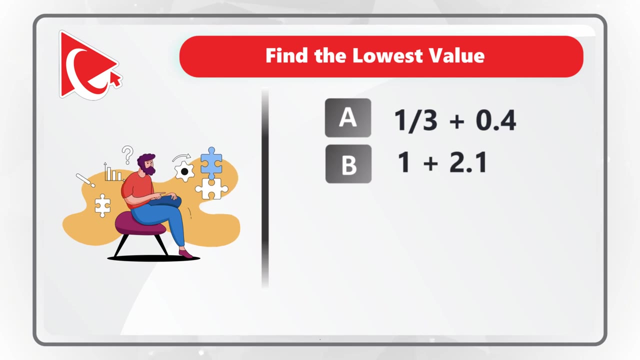 I love this question because it truly makes you think. to determine the final answer, You need to determine which number has the lowest value, And you have four different choices: Choice A: 1 third plus 0.4. Choice B: 1 plus 2.1. 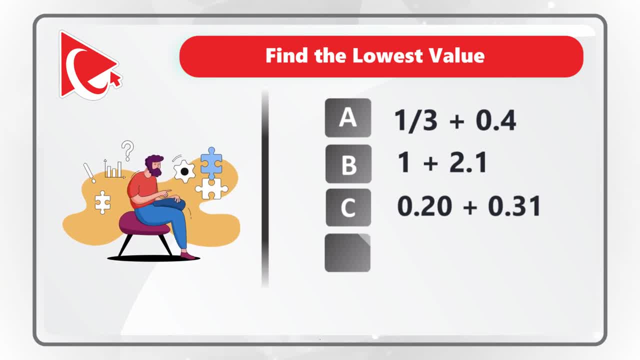 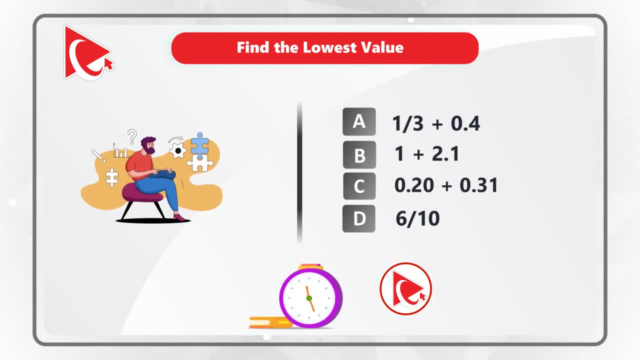 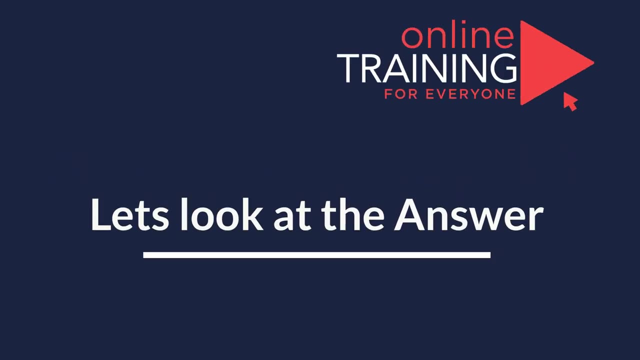 Choice C: 0.2 plus 0.31 And Choice D: 6 tenths. Give yourself a few seconds to see if you can come up with the solution. The tricky part here is that the question is designed to make you do a mental math. 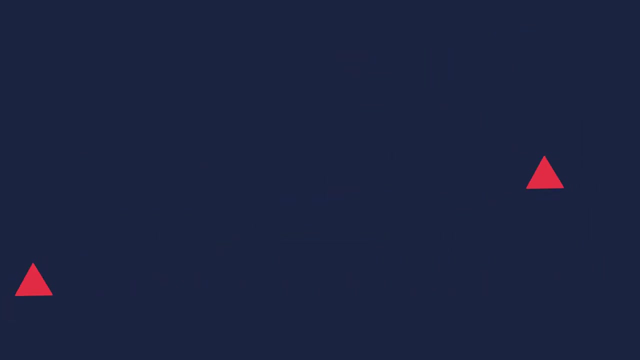 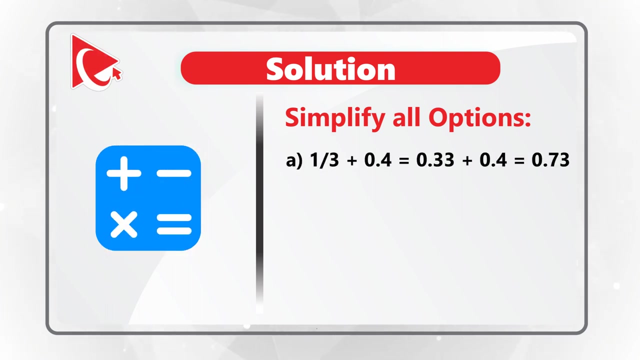 To get to the final answer, you need to simplify all the options. For example, option A: 1, third plus 0.4 equals 0.33 plus 0.4, which is 0.73. Choice B: 1 plus 2.1. 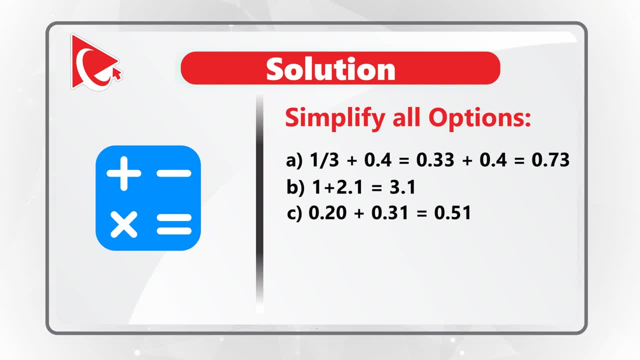 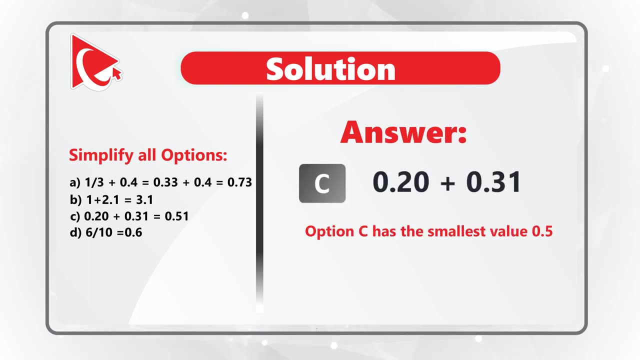 equals 3.1, Choice C- 0.20 plus 0.31- equals 0.51 And Choice D equals 0.6, Which means, if you look at the answers, that option C has the smallest value of 0.51. 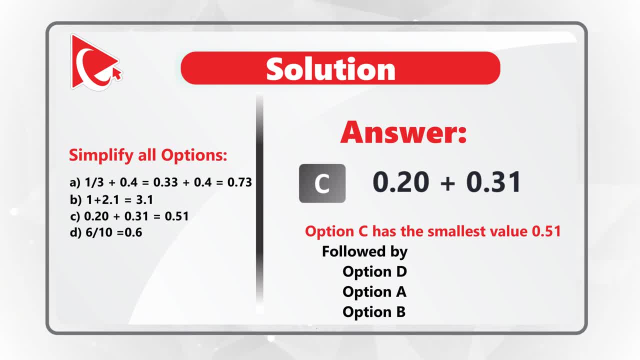 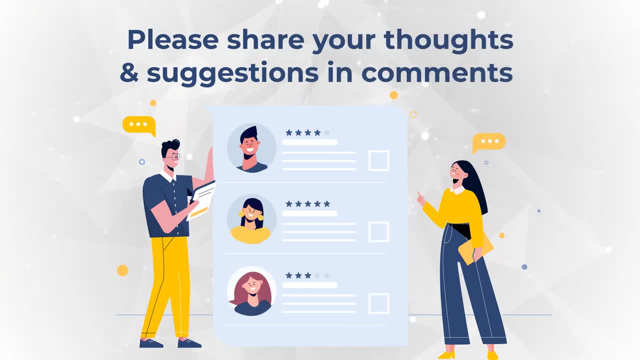 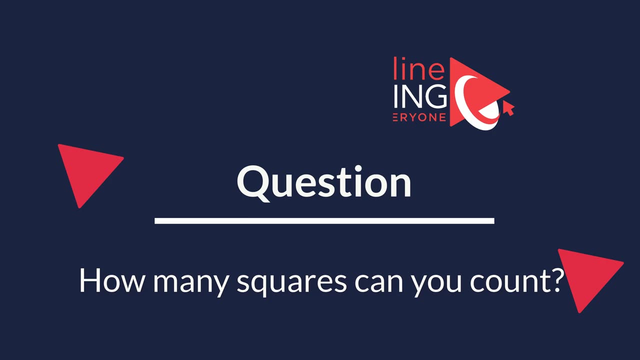 followed by option D, A and B. Was it challenging for you? Please share your thoughts and suggestions on how to better solve it in comments. Here's an interesting question where you need to correctly count the number of squares in a picture. Take a close look. 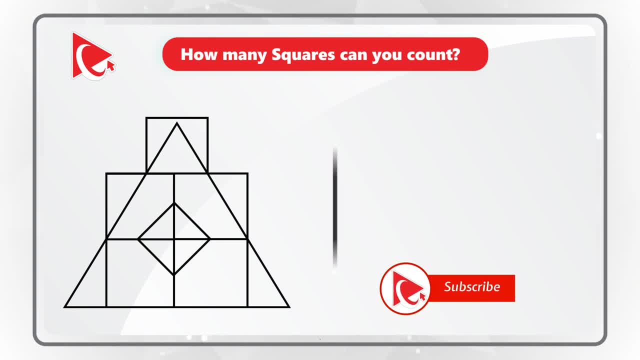 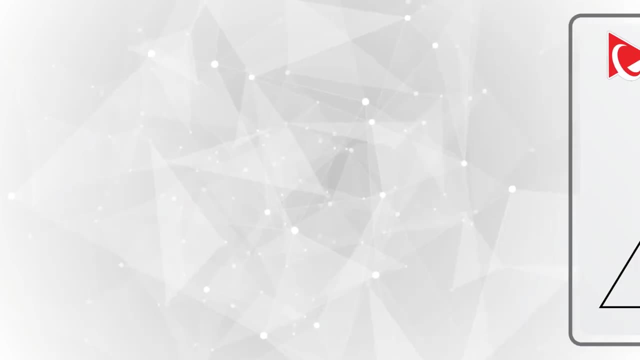 and select from one of the following choices: Choice A- 7 squares, Choice B- 8 squares, Choice C- 9 squares and Choice C- 12 squares. Make sure to count inside and outside squares to get to the correct solution. Let me show you the final answer. 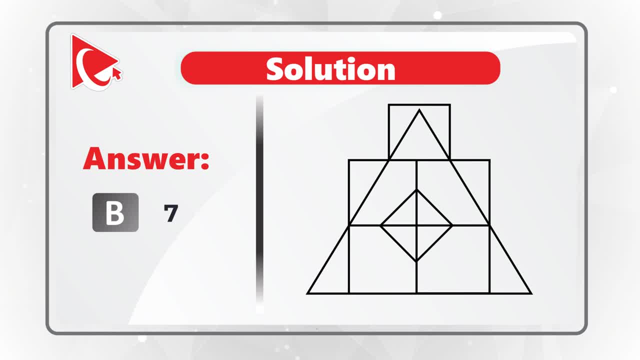 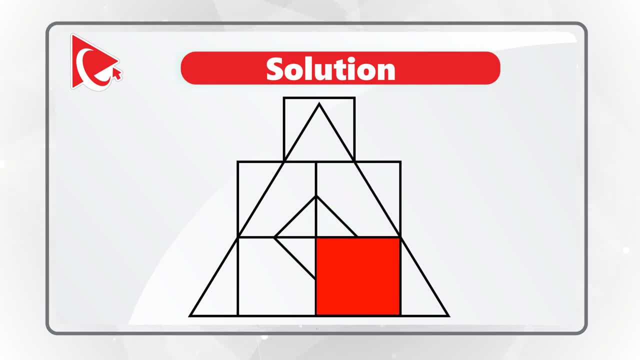 I counted 7 squares in a picture. Obviously, if you have a different answer in comments, here are all the squares: 1,, 2,, 3,, 4,, 5,, 6, and 7.. Do you have a different number? 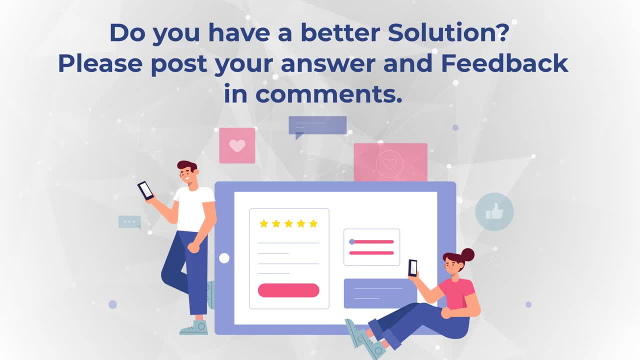 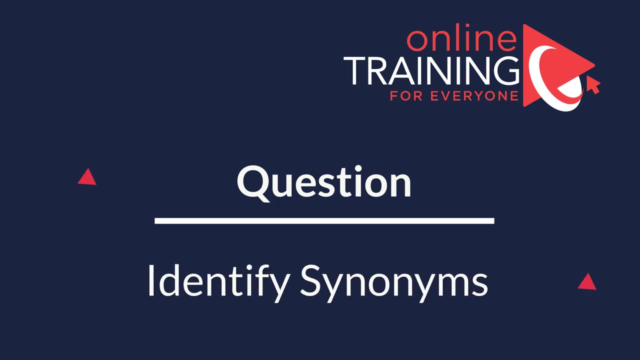 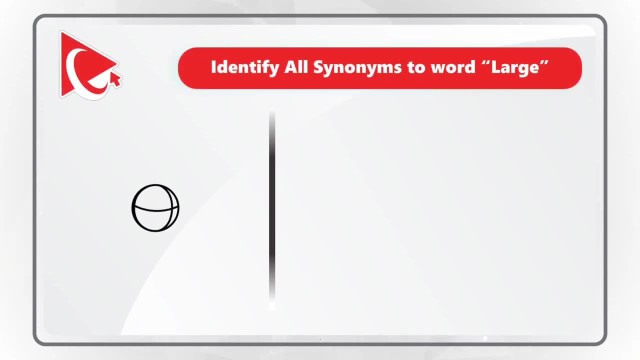 I'm looking forward to your response. if you counted more or less squares? Here's a tricky question which tests your knowledge of English words. You need to identify all the words that are synonyms to the word large. I presented with 10 different words. 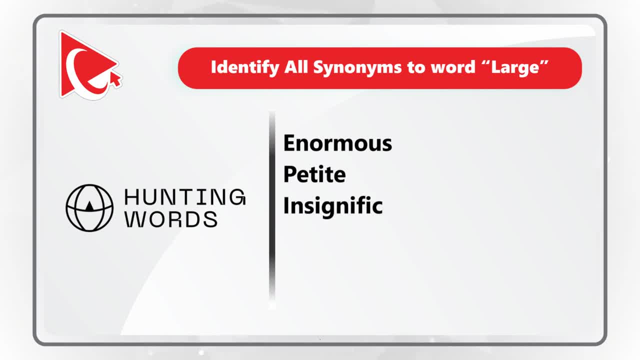 enormous, petite, insignificant, mammoth, minuscule, colossal, huge, powdered, gigantic and dissolved. The tricky part here is that there could be between 1 and 10 answers. Give yourself a little bit of time to see if you can process the question. Feel free to share. in comments. I found 5 words that are similar in meaning to the word large. Let me share them all with you. The words enormous, mammoth, colossal, huge and gigantic are similar in definitions to the word large. Enormous means very large in size, Mammoth means huge, Colossal means extremely large, As well as the word huge has a similar meaning of extremely large. And then, finally, the word gigantic means item of a very large size. And finally, something you may or may not know: 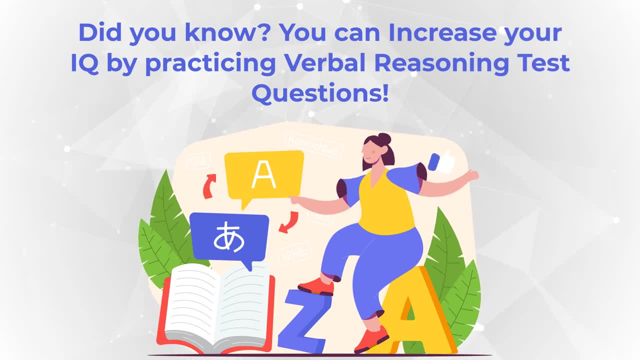 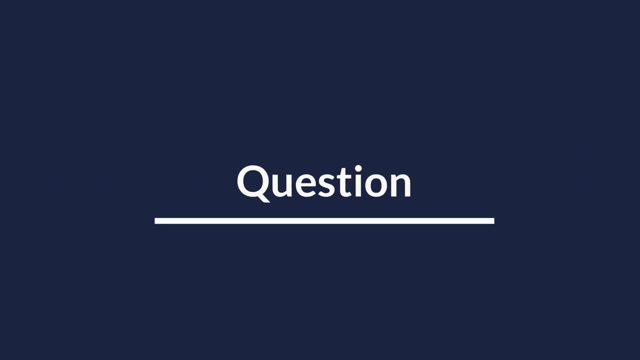 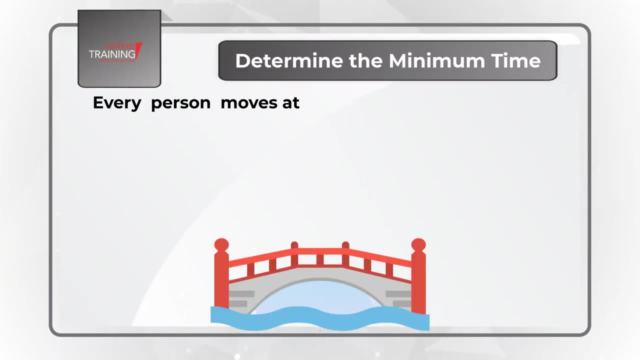 Practicing questions like this not just helps you increase your English dictionary, but also increases your IQ. Here is the interesting challenge you might frequently see on the test. You need to determine minimum time for people to cross the bridge. Every person moves at individual speed. 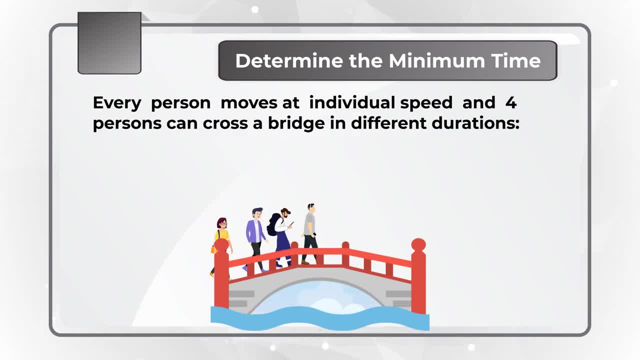 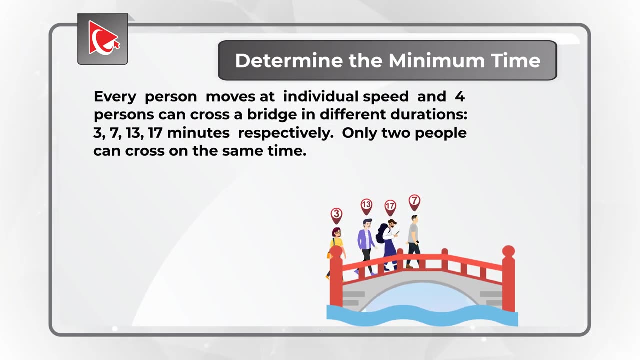 and 4 people can cross the bridge in different durations. They can cross it in 3,, 7,, 13, and 17 minutes respectively. The trick here is that only 2 people can cross the bridge at the same time. You need to determine.